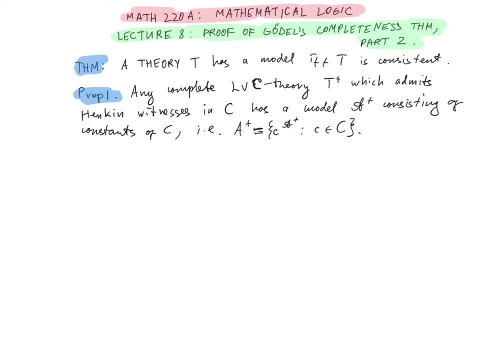 we are able to construct a model satisfying this theory T plus, And then we formulate a lemma which will allow us to reduce the case of an arbitrary theory T, which is consistent to the case of a theory with Henkin witnesses, and complete. 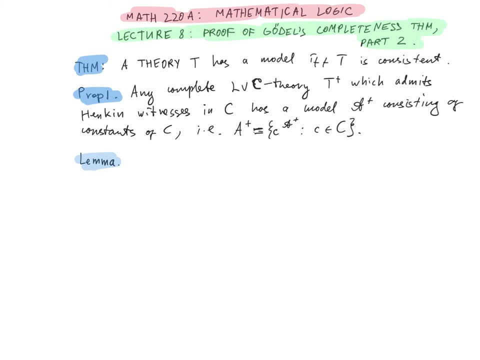 so that building a model for this larger theory T plus will produce a model for the original theory T. The lemma is as follows: For any consistent L theory T, there exists a set of constants, more precisely constant symbols C, disjoined from the language. 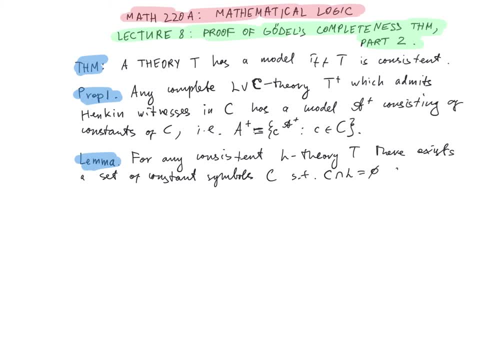 So C, intersection L is empty and such that, taking L plus to denote the language L, union C, there exists a complete L plus, theory T plus, which contains T, and so that it admits Henkin witnesses in C. Now, with this proposition and this lemma in hand, we can conclude the proof of 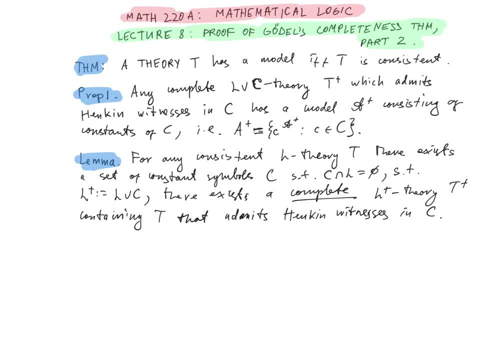 the completeness theorem. So namely, assume we're given a consistent theory T in some language, L, Applying the lemma, we can find a set of constant symbols C- so that explains Expanding the language to L+. containing all these new symbols, we can now find a complete. 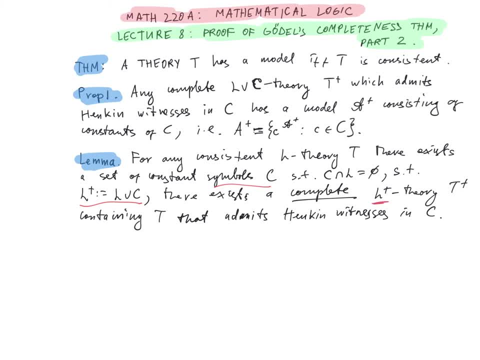 theory, in this larger language, L+, but so that, importantly, this theory extends T and so that T-plus admits Henkin-Witness SNC. Now, by proposition 1, applied to this theory T-plus that we just constructed by dilemma, we can obtain a model A-plus consisting of constants, so that it satisfies all sentences. 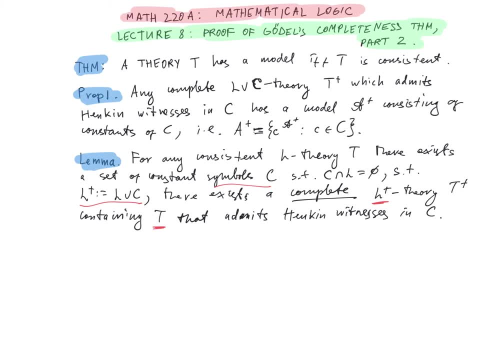 in T-plus, but in particular, since T is a subset of T-plus, it also satisfies all the sentences in T, so it is a model of T as well. More precisely, its reduct to this language, L, which is a sub-language of L+, is a model. 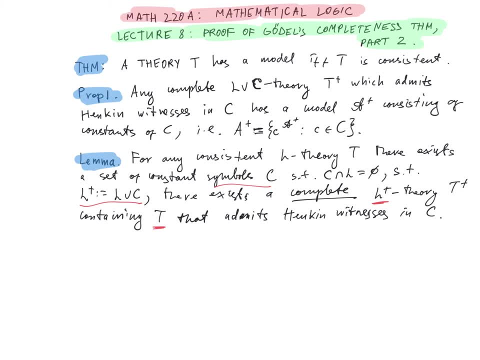 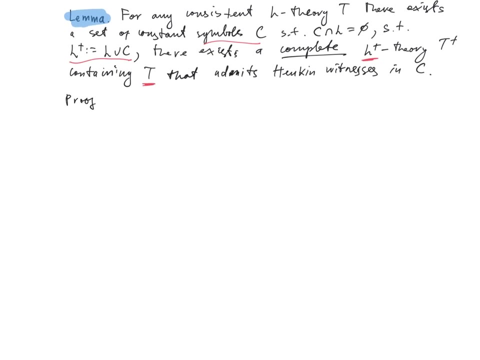 of T. So our aim now for the rest of this lecture is to provide the proof of the lemma Proof to any L-formula phi of X with a free variable X. We assign a new constant symbol, c-phi. now we let c1 be the set of all this constant. 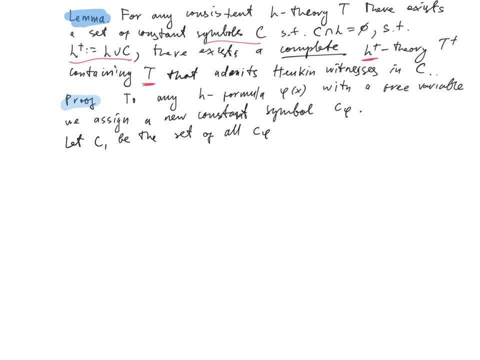 symbols c-phi, a formula with a free variable. we also let L1 be the language consisting of L, together with all the new constant symbols in C1, and we let T1 be the theory, which we will also denote as T tilde, to stress that we are starting with the. 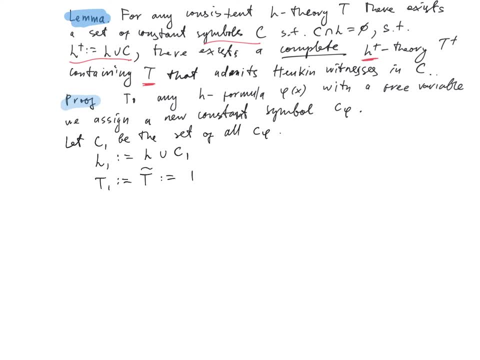 theory T, and we take this to be the theory T, together with all sentences of the form exists x. phi implies phi, with c phi substituting x, where phi of x is a formula of the language L. Next, we claim that the L1 theory T1 is: 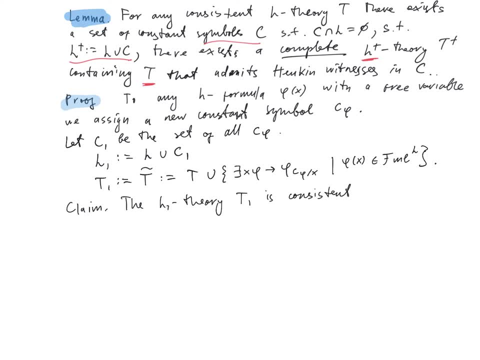 ��고 consistent, or, of course, we assume that the theory T itself is consistent. we know that a theory is consistent if, and only if, any finite subset of the theory is consistent, simply because a proof of a contradiction would only use finitely many sentences from: 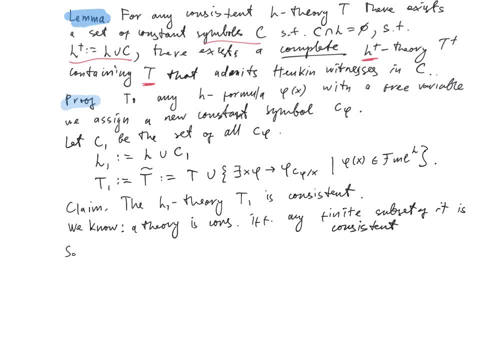 the theory. So it suffices to prove that the theory T tilde prime consisting of the theory T together with all sentences of the form exists. Xi phi i implies phi i with C phi i. substituting Xi i less or equal than n is consistent for any finite. 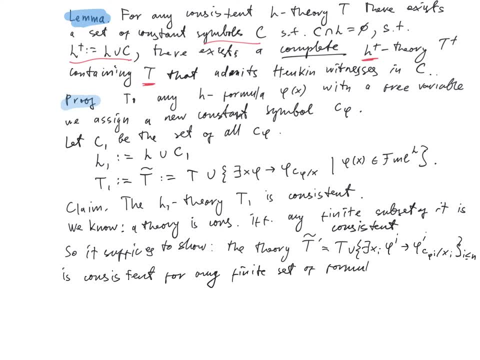 set of formulas in the language L, So finite set of formulas, phi i through phi n. Now note that the theory T is consistent as an L-theory implies that T is also consistent When viewed as an L-prime theory. this implication holds by the simulation of constants by variables. 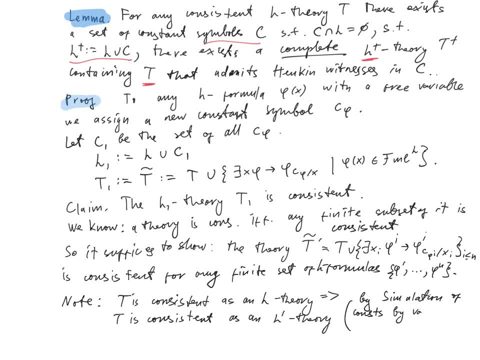 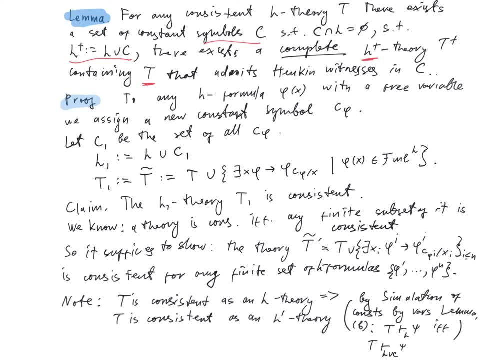 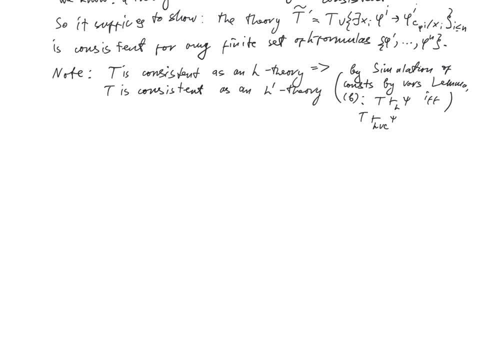 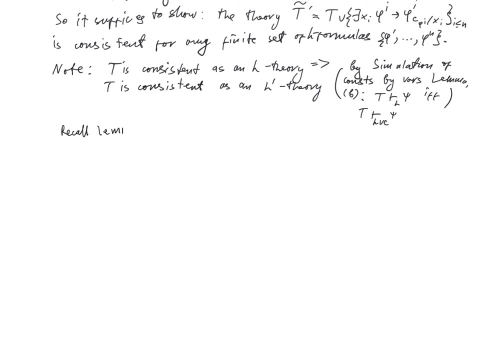 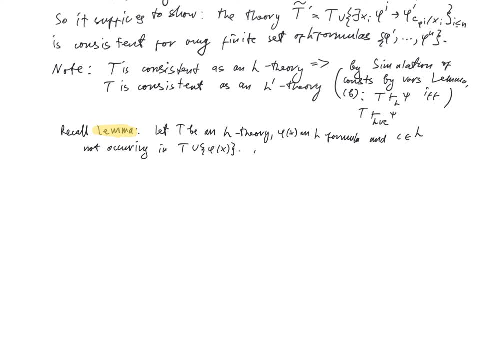 union phi of X. Assume also, Let's do it again, Assume also. Assume also that T is consistent, then we have that T union. the sentence exists as phi implies phi with C substituting X is a consistent L-theory. 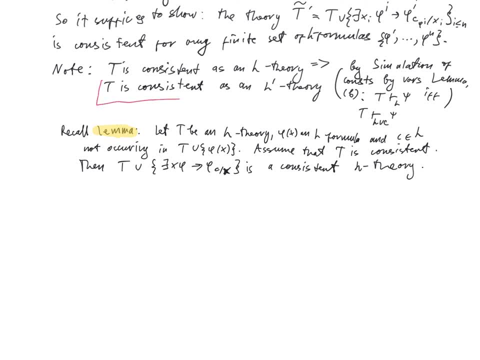 Now note that, Since we know that T is a consistent L-prime theory, if we only had a single formula phi one that we were trying to add to the theory T while maintaining consistency, this would follow immediately from this lemma. But also after adding a single formula phi one, we can now consider this new theory consisting: 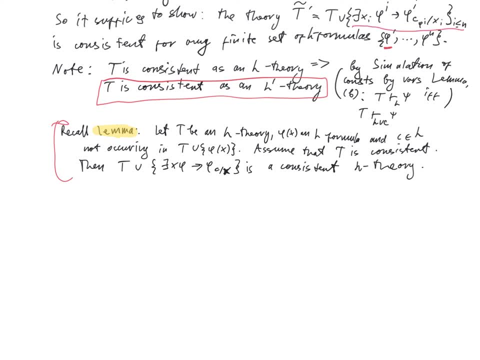 of T together. We can now consider this new theory consisting of T together with the corresponding sentence for the formula phi one and apply the lemma again to this extended theory and the formula phi two, again obtaining consistency, And we can repeat this process and steps one by one, inductively using the lemma in order. 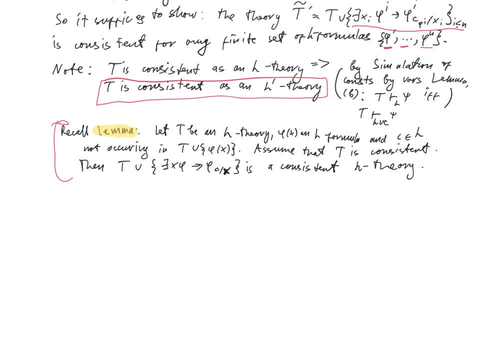 to conclude that the theory T, tilde prime, With any finite set of formulas phi one through phi n is consistent. well, together with the sentences of this form corresponding to the formulas phi one through phi n is consistent. And so, by the previous remark, since we only need to check consistency for finite subsets, 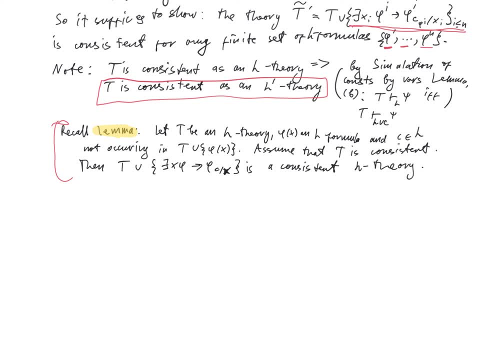 of a theory, we conclude that the theory T tilde itself is also consistent. So T tilde prime T tilde is consistent, Which, recall, also correspondent to the theory T one. So next we are going to iterate the construction With C two. 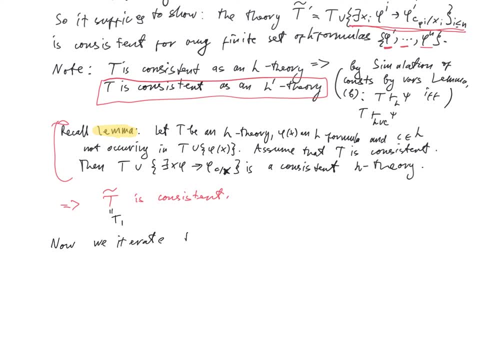 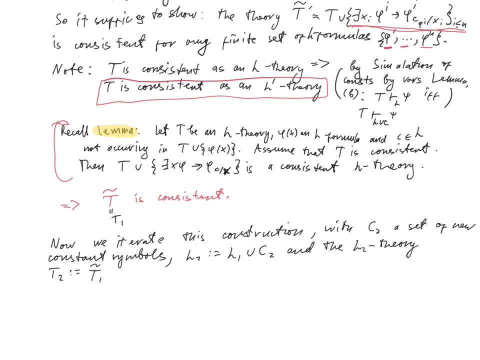 take to be T one tilde tilda. so we have to add sentences of the form t1, so we have all sentences from t1, and we have all sentences of the form exists x phi implies phi, with c phi substituting x. 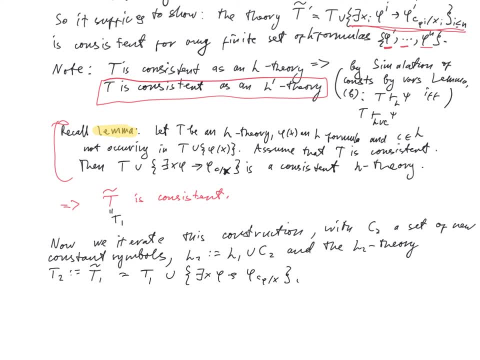 where phi varies over all formulas. but now of the language L1.. Repeating the same argument as we just gave with respect to t1 instead of t, we conclude that t2 is also consistent as an L2 theory. and then, by induction, 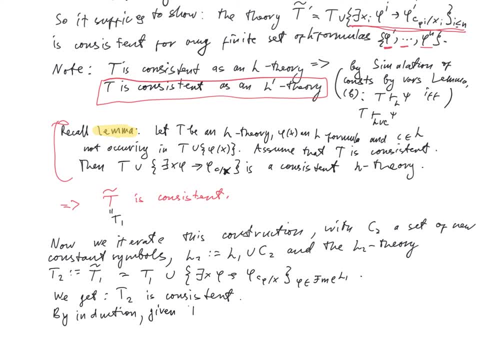 given some theory: tn in a language ln, which is formed using a set of constant symbols, cn. we define a new set of constant symbols, cn plus one which consists of all new constants of the form c, phi, where phi is a formula with a single free variable in the language ln. 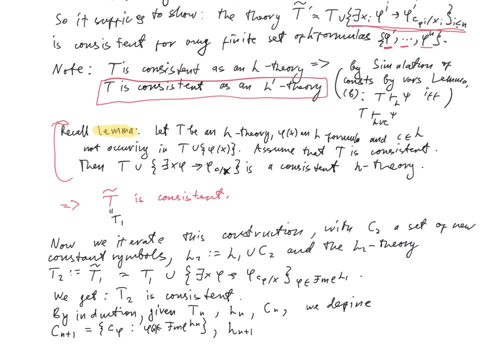 Then we define the language Ln plus one to be the language ln, together with this new constant symbols, And we define the theory T to be the tilde operation applied to the theory T. So note that T is an L theory, which is, moreover, by the previous argument. 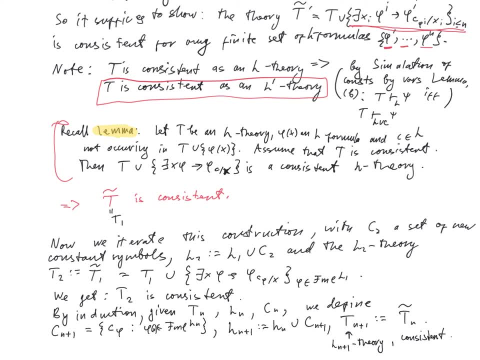 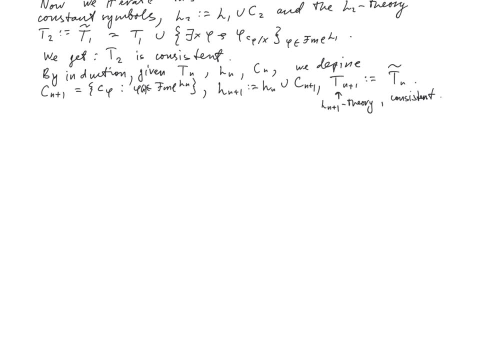 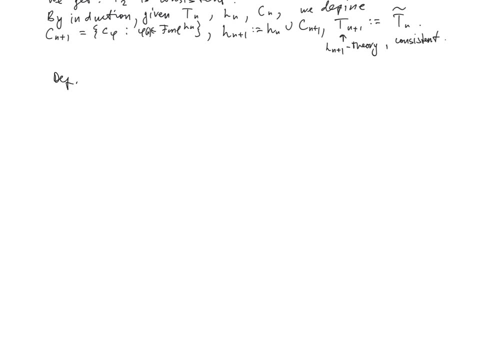 is consistent. Now we want to consider the situation in the limit. So we define C to be the union of all of this set of constants, Cn for n varying over the natural numbers, And the language L plus to be the language L union C, so it's a language which contains 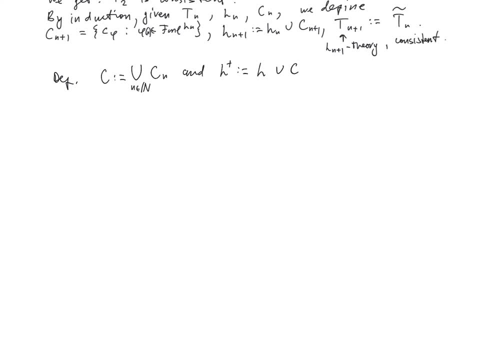 all these constant symbols added on each of the countably many stages of the construction. Then we have a sequence of theories- Tn for each natural number, n- which forms an increasing, in the sense of inclusion, sequence of consistent L plus theories. Then we know that the L plus theory, T prime, which we take to be the union of all of the 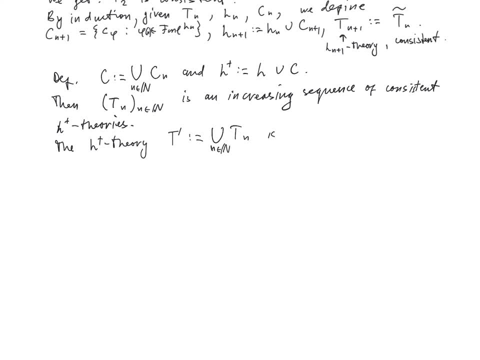 theories. Tn, A natural number, is also consistent as a union of an increasing sequence of consistent L plus theories And finally by construction, it admits. Henkin witnesses in C Indeed note that given a theory Tn at the stage n, the definition of Tn tilde which 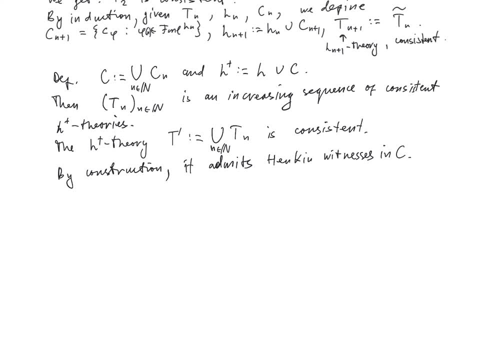 we took to be Tn plus 1, ensures that we are explicitly adding sentences, all of the sentences that are needed to ensure that all formulas from Tn are consistent. So we have a sequence of theories, Tn And finally, by construction, it admits Henkin witnesses in C. 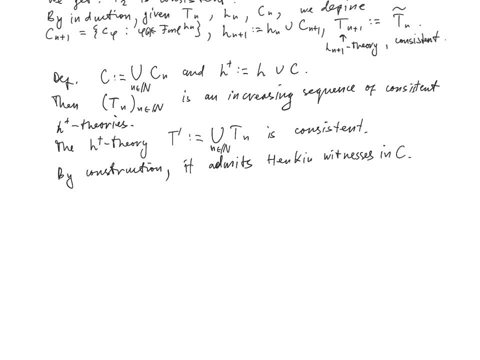 Rather it brings together Tn andские mujer, and we are free from the units such as a union of all branches, juily formed from the union of a series Tn. All triangles from Tn have a Henkin witnessахin the theory Tn plus 1.. 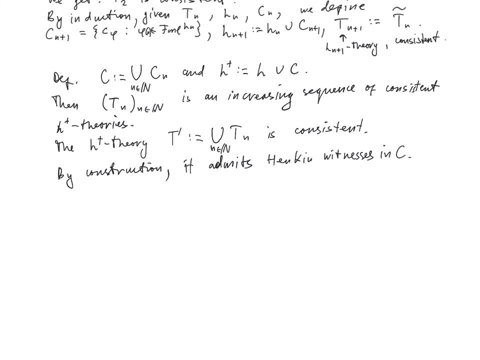 So on each stage, Henkin witnesses are added at the next stage. and since we are taking, And so of course T' also contains that formula, So T' is closed under adding formulas required in the definition of admitting Henkin witnesses. And so T' admits Henkin witnesses in C, the set of all the constant symbols added on all. 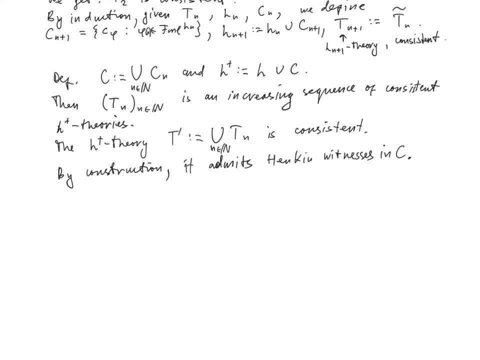 of the stages. This way we have obtained a theory T' which extends T and admits Henkin witnesses in a new set of constants C. So what is missing to get the full result of the lemma is the question of whether T' is complete or not. 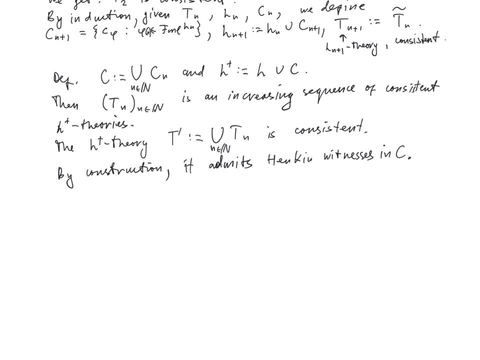 A priori, it has no reason to be complete. and so, on the next stage of our construction, we are going to ensure completeness by considering a larger theory, potentially. And so, on the next stage of our construction, we are going to ensure completeness by considering a larger theory, potentially. 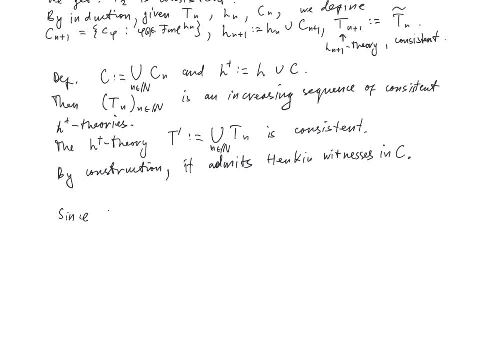 So since any L' theory S' containing the theory T' still admits Henkin witnesses in C, So since any L' theory S' containing the theory T' still admits Henkin witnesses in C. Indeed, we are not adding anything more to the language, so S prime is in the same language. 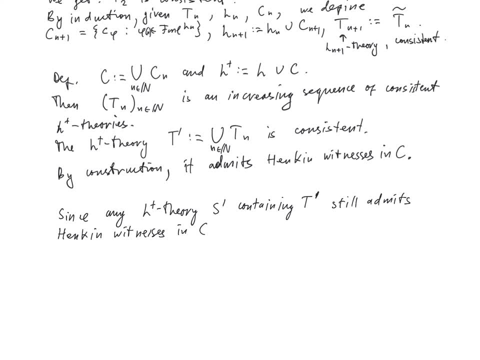 L prime and, by the assumption, T prime already contains a formula for each L prime formula. phi T prime contains a formula saying that it has a hand-kin witness in C, And so, since we are only adding more formulas, any S prime will also contain all of these required sentences. 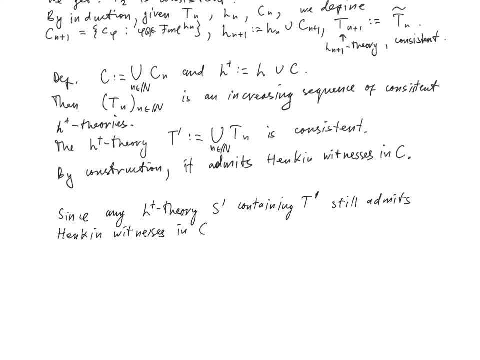 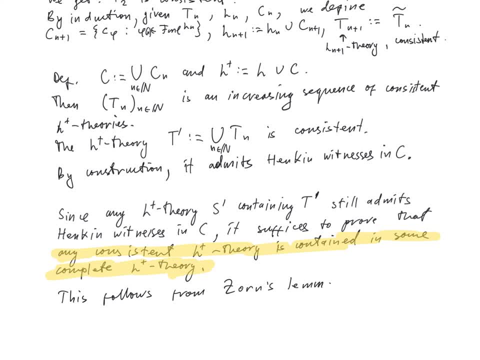 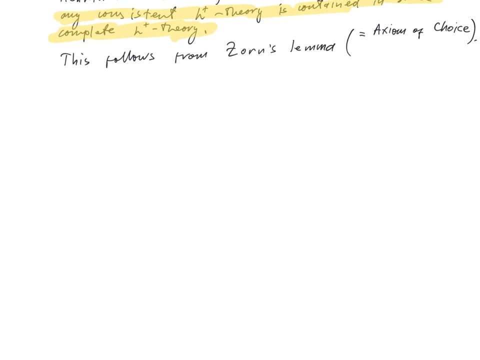 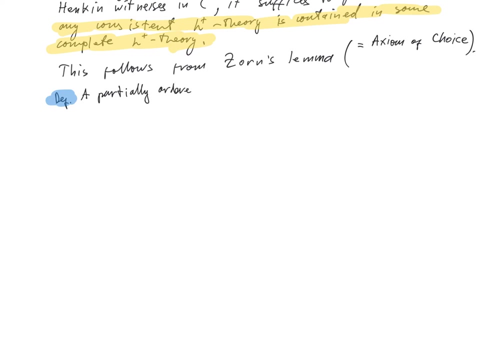 Which is, of course, one of the equivalent formulations of the axiom of choice. Definition First, a partially ordered set X is said to be inductive if any totally ordered subset Y of X admits that any totally ordered set A is equal to any totally ordered set Type. 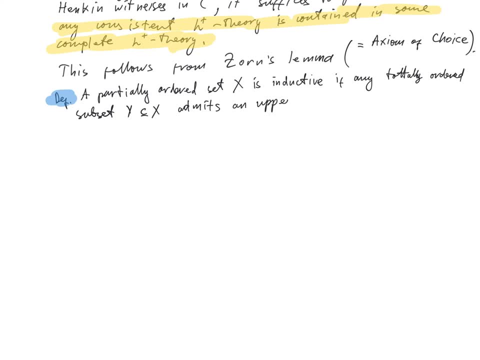 Next, some sort of revolution means that we have an absolute possible setaji, and here we have an absolute possible set. hoje Does not say that, in fact, And one can use this curve, One can use this freshman idea: Say: for every B, we add one set. A to the trapezoid, one set, Z to the trapezoid, one set. X to the trapezoid. An answer is that two set, A compared to可愛, B is less than or equal than A to the trapezoid of the set, Y is хX and such like, A is less than or equal than x. 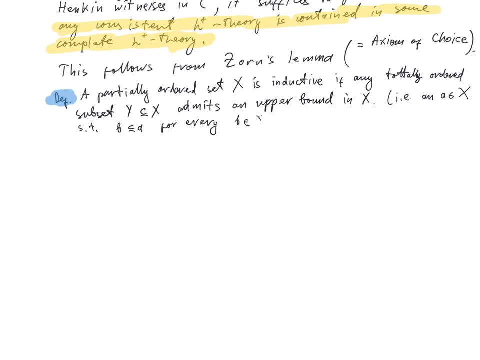 So there Heck again. work in common sense. So we do not want anyone to worry about the fact that. let me explain the reason we are introducing 1 and h and H of x B in Y. Note that this implies in particular that X itself is non-empty. 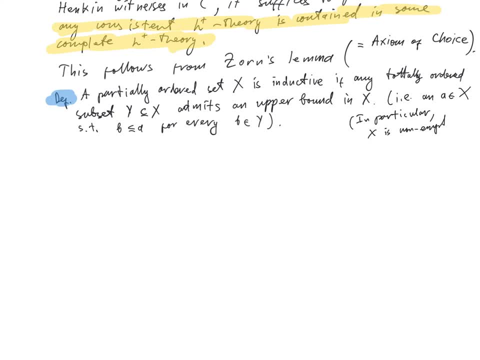 Now Czorn's lemma, one of the brilliant reformulations of the axiom of choice, along with the well-ordering principle and many others- says that every inductive partially ordered set is a non-empty. This means that every inductive partially ordered set admits a maximal element. 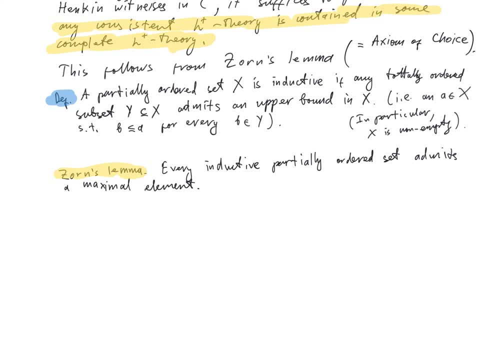 We will see that Czorn's lemma allows us to show that every consistent theory is contained in some complete theory, which is exactly what is needed to finish the proof of the completeness theorem. For this purpose, we consider the set S of all S' containing T', such that S' is a consistent. 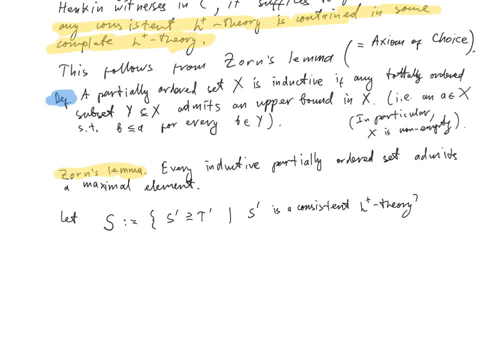 L-plus theory. Note that there are at most two to the cardinality of the language, L-plus theories in this language. So in particular, this is a well-defined set. Now we note that this set is non-empty, since it contains the theory T' itself, which we 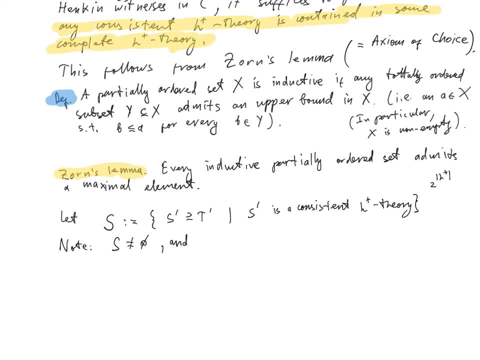 know is consistent. Note that there are two to the cardinality of the language, L-plus theories. in this language We know that bets. This set is unopposed to the principle code And this set is also partially ordered under inclusion, In this case heheads. 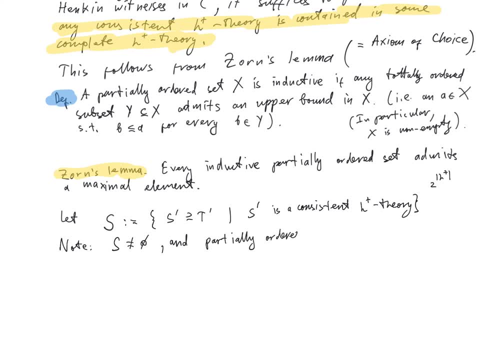 This set is non-empty And we also know that the union of the very positive values is possible under the L's literal order. Now we have one drapery that is now under inclusion, Preforwardly some more years in this case. 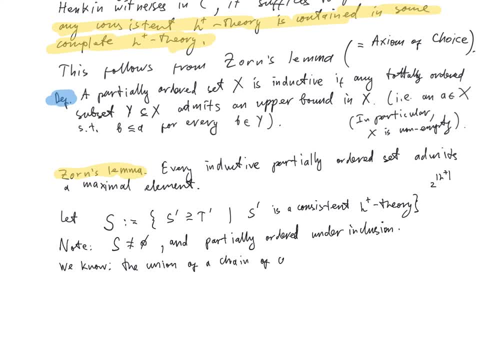 Here. this is the solution. And now a set of numbers coming under inclusion, Worth of the opposite of the first set of the union in terms of considered values. and this of consistent theories is itself consistent. hence this ordering on S is inductive that there exists a maximal element in S. 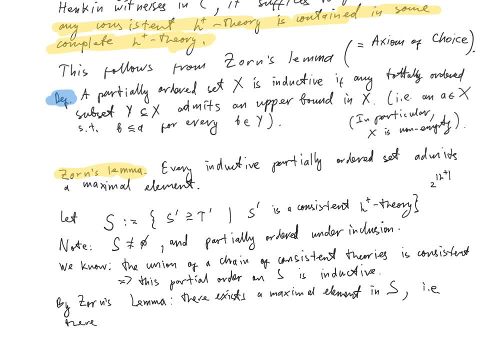 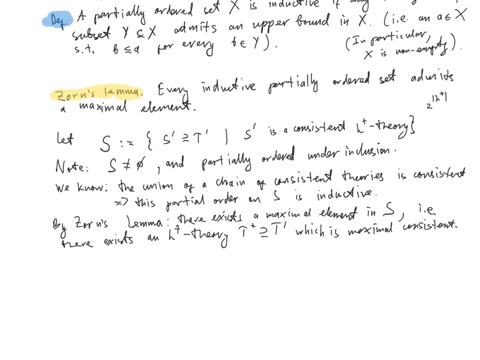 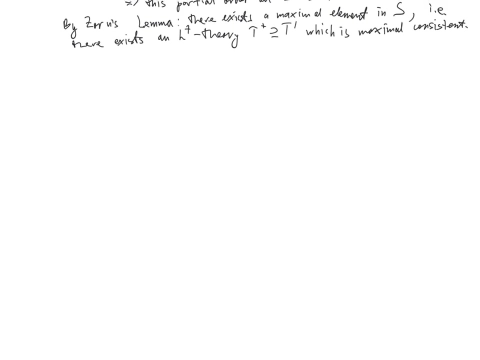 that is, there exists a maximum element in S. that is, there exists that there exists a maximum element in S, an L plus theory, T plus containing T prime, which is maximal consistent. Now our task is to show that this theory is complete. towards this purpose, let phi be. 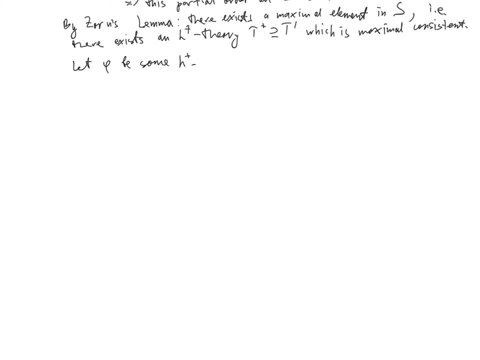 some arbitrary L plus sentence and assume that T plus does not prove phi In the sense of the language L plus, then we know that the theory in the language L plus, consisting of the theory T plus, together with the negation of phi, is consistent by 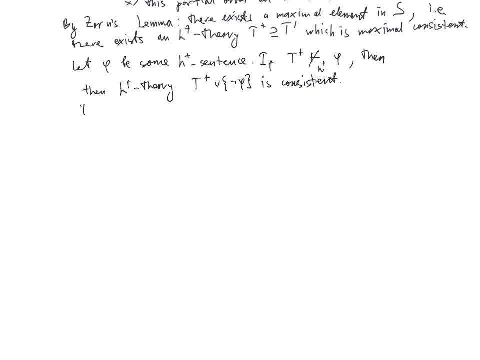 a corollary of deduction lemma. But then we conclude that not phi must belong to T plus by maximality, since T plus is a maximal consistent theory already. hence we get that T plus is complete. Thank you, And this finishes the proof of the completeness theorem. 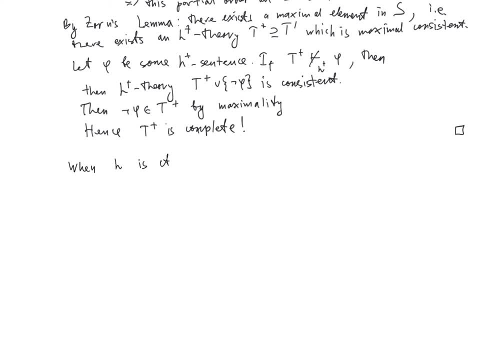 When the language L is countable. we can provide a more direct argument For the theory in the lemma as follows: We fix a set C of countably many constants in the theorem and simply apply Lincoln's CN and a natural number of new constant symbols and we enumerate the set of all L union C. 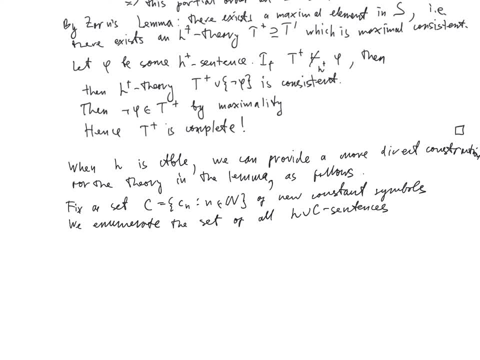 sentences, which is of course countable in an arbitrary manner as phi 0,, phi 1,, etc. So we fix some enumeration, then by induction we construct an increasing sequence: TN with n, a natural number of consistent L, union C theories with the following properties: 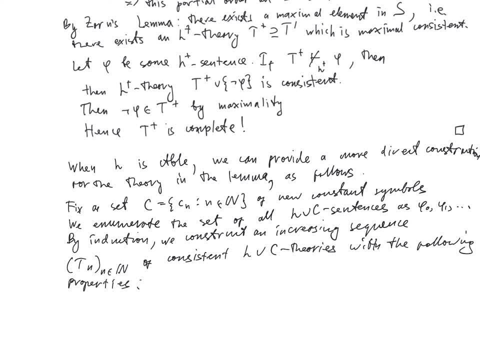 So this, the first theory in the list T0, is the original theory T, and we also have that TN minus T0 is finite for any n. So on each stage we're only adding finitely many new sentences. We also have phi n belongs to the theory TN plus 1, or its negation. not phi n belongs. 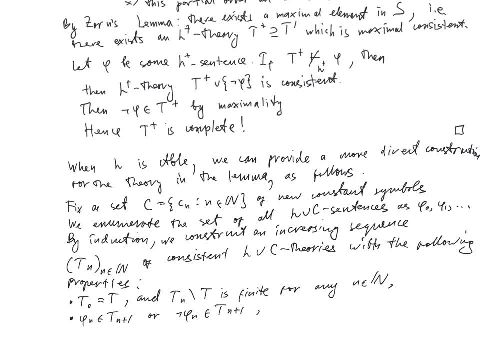 to the theory TN plus 1.. So the sentence phi n gets decided on the stage TN plus 1, and we also require that if phi n is of the form n, If there exists x psi, for some psi belongs to TN plus 1, then there exists a constant. 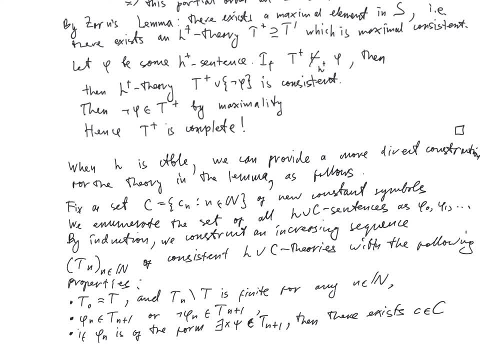 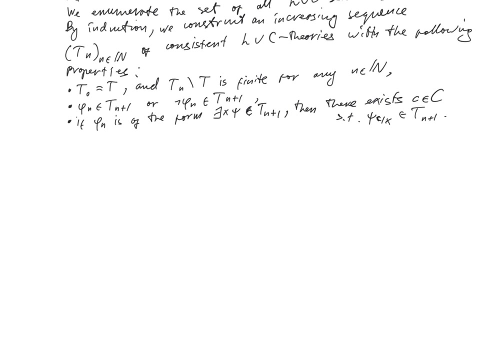 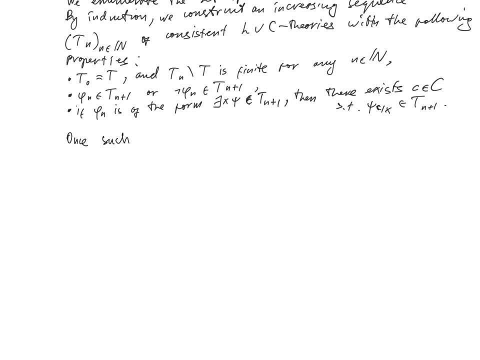 symbol C in the set of constant symbols, capital C, such that the formula psi with C equals n plus 1.. So this many clever solutions. So again we've 3000 abstract terms. for all of them, And if phi n equals x psi, into the summation of a comma we just need to add n to that. 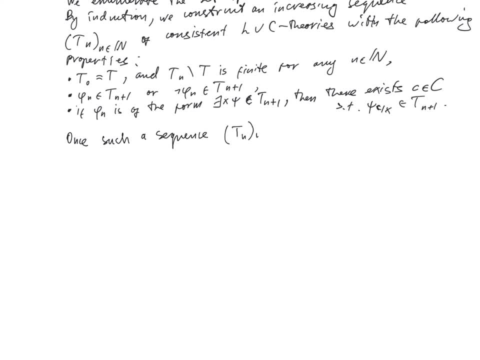 name element. so with the missing constant, add the first step�: fug in theถ. Uhh, finishing, the set of no's for x psi is n plus 1.. And this given, Then it is enough to set T plus as the union of the TNs, because then we have that T plus. 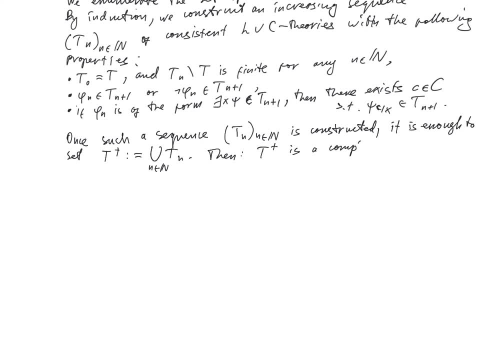 is complete theory by construction, because we know that each of the sentences appears somewhere in the enumeration, and as phi n, let's say. and then we know that on the next stage, the theory TN plus one contains either phi n or its negation. 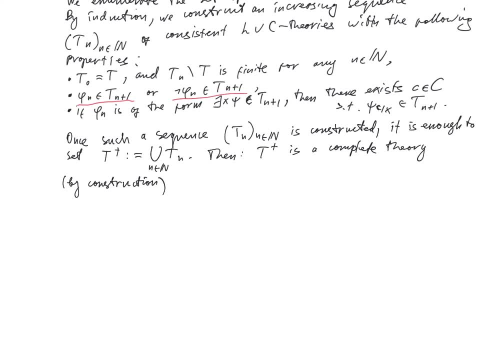 Okay, Okay, Okay. And we also know that T plus admits Henkin witnesses in T in C. excuse me, so why does this hold? So to see this, consider some L union C formula psi of X with the free variable X. then there exists some natural. 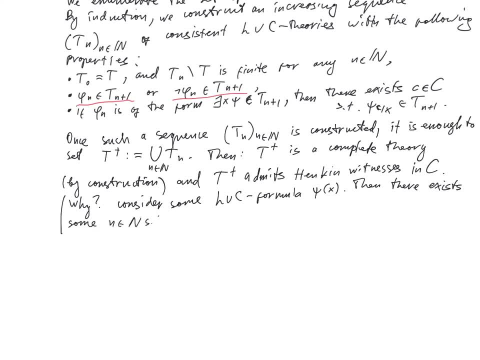 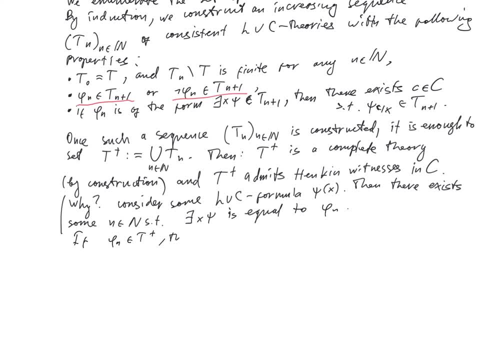 Okay, Okay, Okay. So let's go to the sentence phi n in our enumeration of all sentences. Now, if phi n belongs to T plus, then by construction we have that psi with C substituting X belongs to T plus, Okay. 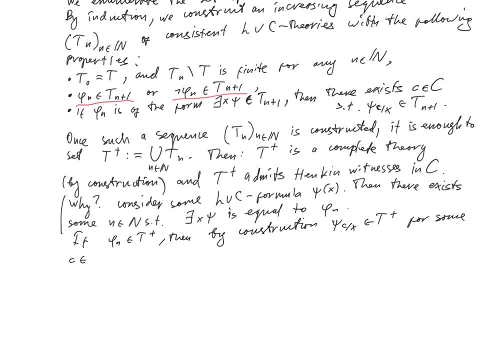 Okay, Okay, symbol C in C, and hence we also have that exists X Psi implies Psi with C substituting X, so this sentence belongs to T plus as well. otherwise we have that the negation of exists X Psi belongs to T plus. hence we have that the sentence exists X Psi implies Psi with. 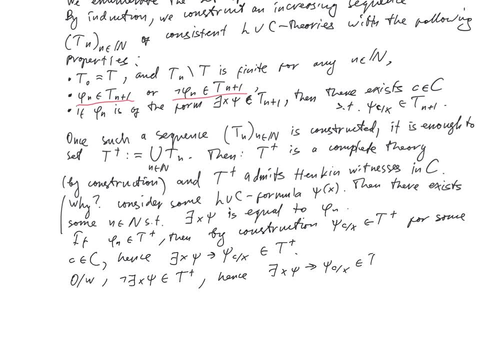 C. substituting X belongs to T plus for any constant symbol C in C. So together this shows that the theory T plus and meets Henkin witnesses in C. Hence, if we can carry out the inductive construction of the theories Tn with these three properties, then we also get: 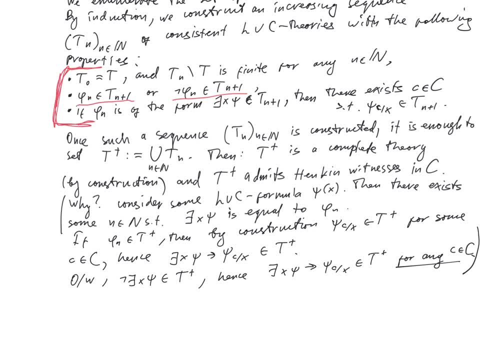 a complete theory with Henkin witnesses, and hence we find a model for the original theory T. So now let's explain how to get this inductive, how to define this inductive. theories Tn. So assume that Tn is already constructed of. 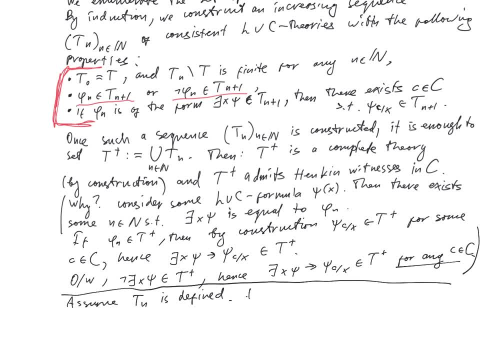 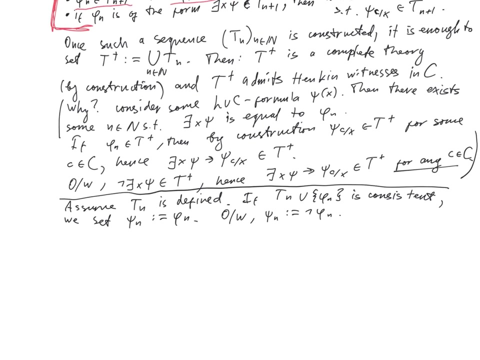 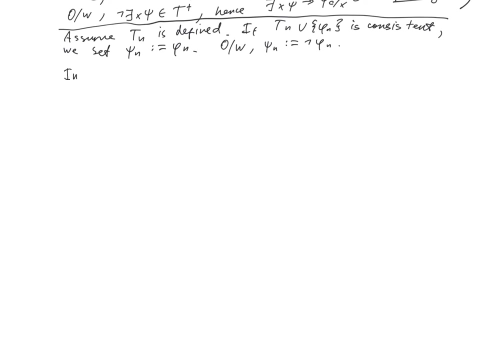 course, the base case being T0 equals T. Now, if the union of Tn with phi n is consistent, then we set Psi n equal to phi n. Otherwise we set Psi n equal to the negation of phi n. Then in both cases, 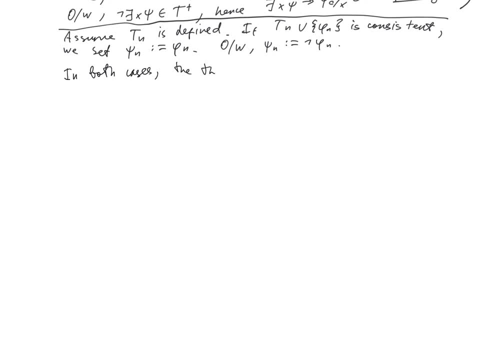 the theory Tn together with the sentence Psi n is consistent. Now, if Psi n is not of the form exists x chi, we set Psi n equal to the negation of phi n. Now, if Psi n is not of the form exists x chi, we set Psi n equal to the negation of phi n. 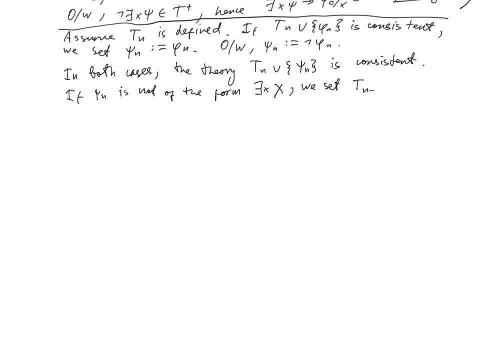 Then, in both cases, the theory Tn plus 1 to be the theory Tn, together with the sentence Psi n. Otherwise, we let m be minimal, Minimal natural number, such that the constant symbol Cm has no occurrence in tn and we are guaranteed that such nm exists, since we know that tn minus t is finite. 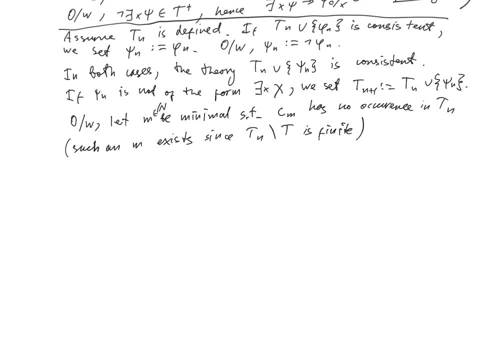 because, remember, on each step, by the inductive assumption, the difference is finite. we only added finitely many sentences, and here we only have n steps, so altogether n steps from the theory t0, so altogether we only added finitely many sentences. hence this difference. 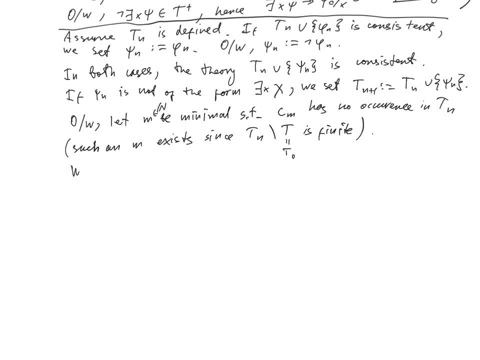 is finite, then we set tn plus 1 to be equal to tn, together with the sentences psi, n and also chi, with cm substituting x. Then the theory tn plus 1 is consistent, again by a lemma that we have proved in the previous. 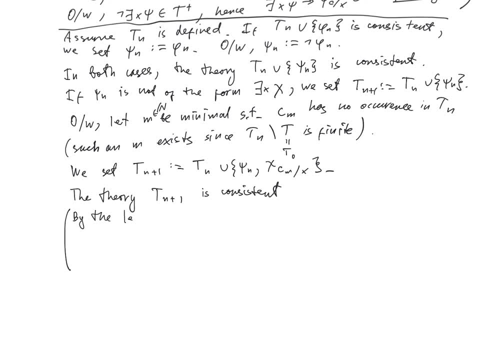 lecture. It says that if t is consistent, then also t, together with the sentence exists x, phi implies phi with c substituting x is consistent under some assumptions which are easily satisfied in this situation. So this gives This sketch, provides an argument, a more constructive argument in the case of a countable language. 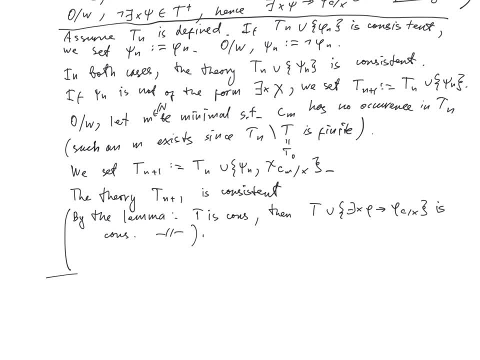 when the theory t is in a countable language, L. Let us conclude with a small foundational remark, since we already saw that Sorn's lemma allows us to prove the completeness theorem For theories in languages of arbitrary cardinality. It is also known that the general form of the completeness theorem 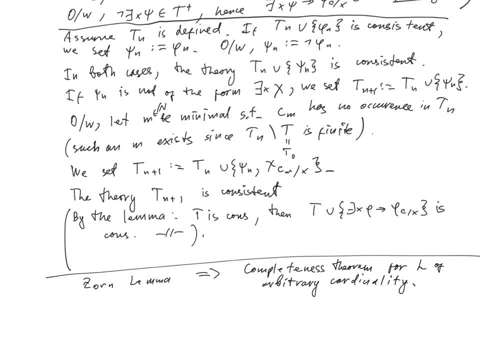 completeness theorem for languages of arbitrary cardinality implies a weak form of the axiom of choice, the so-called ultrafilter lemma, which is also sometimes referred to by the dual name of the prime ideal. lemma, which guarantees existence of prime ideals, or 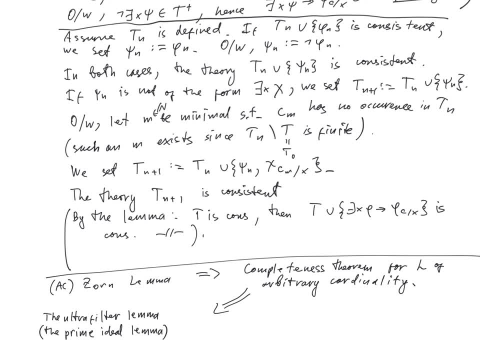 respectively non-principal ultrafilters in Boolean algebras. So this is again known to follow from the axiom of choice and the converse implication is not true. There exists models of set theory which only satisfy this weaker form of choice, but not. 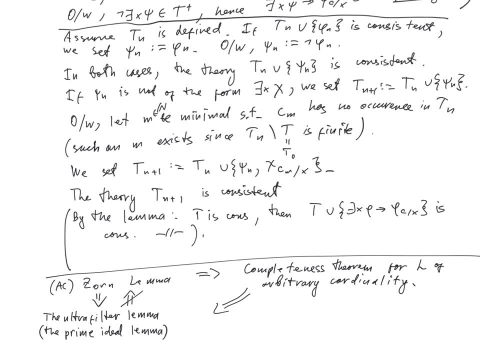 the full axiom of choice. And finally, we saw that the completeness theorem for countable languages is provable only in the set theory. And finally, we saw that the completeness theorem for countable languages is provable only in the set theory. And finally, we saw that the completeness theorem for countable languages is provable. 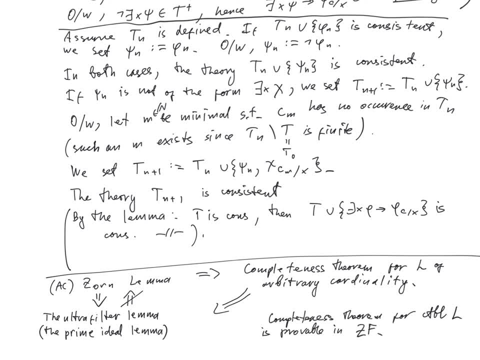 only in the set theory. And finally, we see that the completeness theorem for countable languages is provable only in the set theory. And finally, the completeness theorem for countable languages also results in ultrafilter lemma. we've concluded here with this foundation remark, since this is not the main topic of